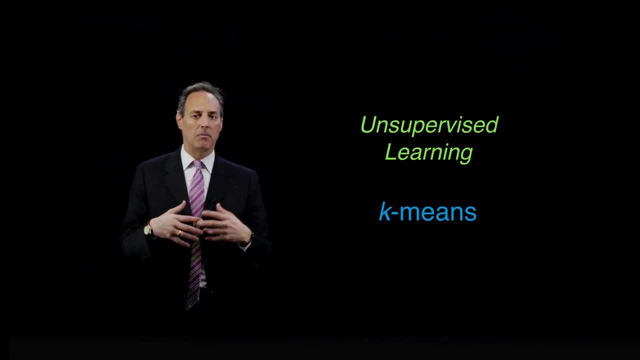 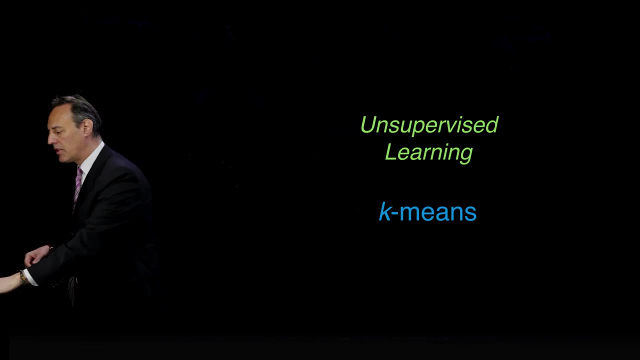 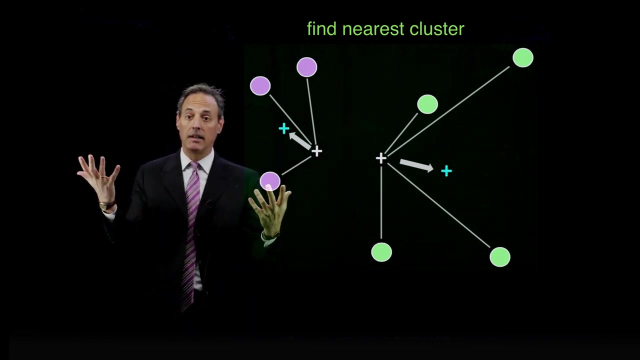 and also when you're trying to extract features out of that data to make meaningful decisions. OK, so what is k-means and how do we use it? So the k-means algorithm is pretty simple to understand. You're just basically going to say: take some data, it's unlabeled and 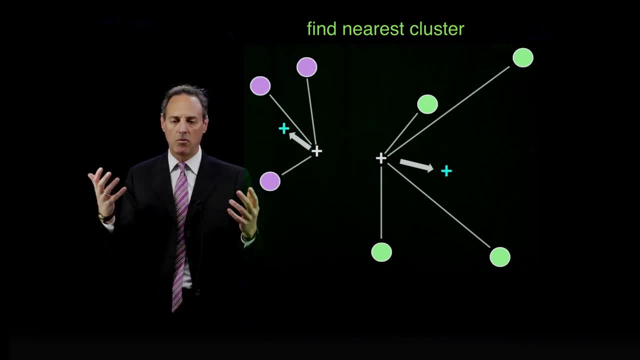 in fact I've colored those balls here, but initially the balls would just have no label whatsoever, and the idea behind k-means is that you pick how many clusters you think are going to be in your data. So this, this is interesting. the selection of of the next. two is K-means right? Because it's. if you take this bunch and drill this K-means extra things, that won't work, and I could grind it in just a few minutes. In fact. this is quite simply for a lot of you, this model is crazy. This is when it's easy to see you're no longer. 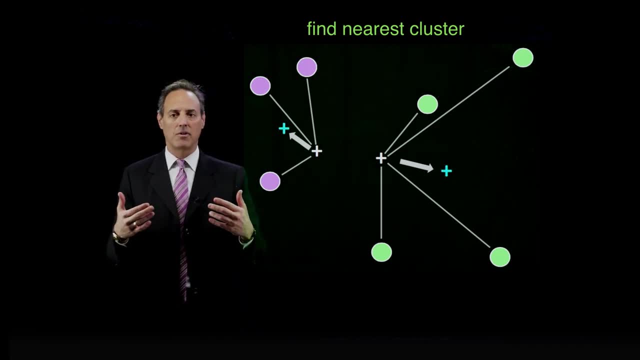 learning and understand episode number 2.. So I'm going to show some things from the longtemps. The number of clusters, to begin with, is already sort of a supervision portion of this that you would have to provide. However, you can also start thinking about picking different cluster sizes and pruning it if it's too many. 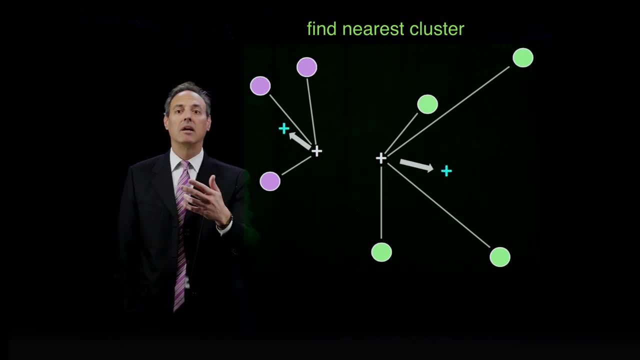 or growing it if it seems too few, depending upon how you think your algorithm is actually doing and how many distinct clusters you think you might have in your data. Here the idea is in this little picture I'm showing you. I have some data and I want two clusters. 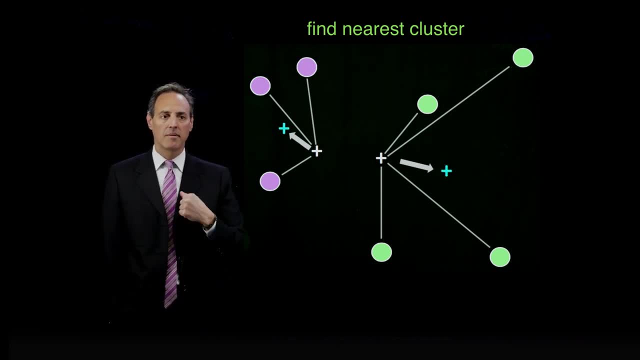 So what you would initially do is pick two random points. So those are denoted here by this plus sign here in gray, this plus sign here in gray here. So I just pick two points and I say those are the centroids of my two clusters. 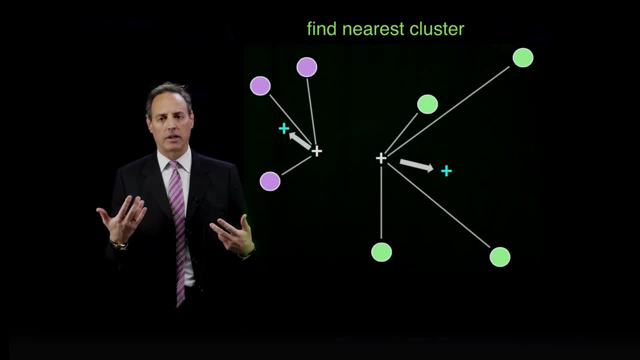 Of course I've just guessed, so I have no idea if I'm correct or not. In fact there are no labels, So it's very hard to tell if the truth has been achieved anyway. But those are the two points, And then what I do is you simply take every single data point and you find the nearest centroid cluster. 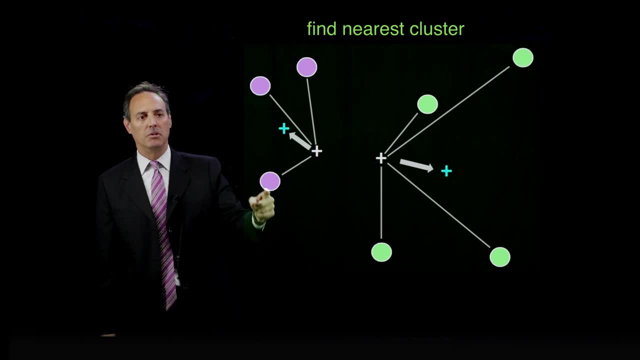 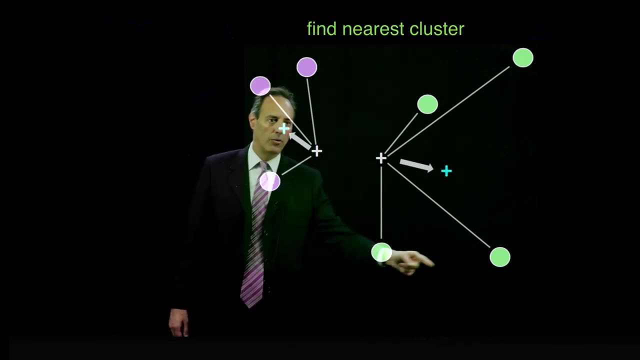 So this is why I've labeled all of these balls here to be magenta, because they are closest to this magenta point. Here. the green balls: they weren't green, they were gray, but I turned them green because they are close to. 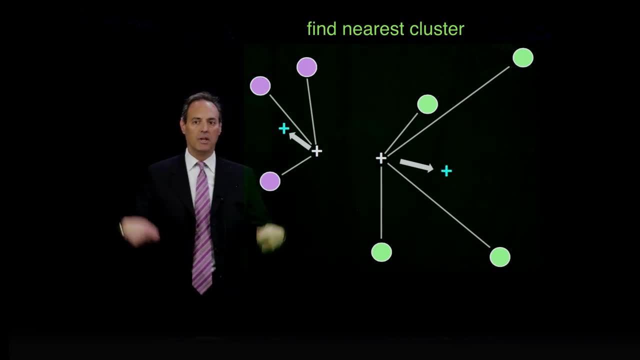 So I'm going to take this cluster- That is step one of the algorithm- Pick two initial points. Every point just goes to the nearest centroid. Now what you do? you look at all the data associated with this centroid and your next point is you go to the center of mass of this data set. 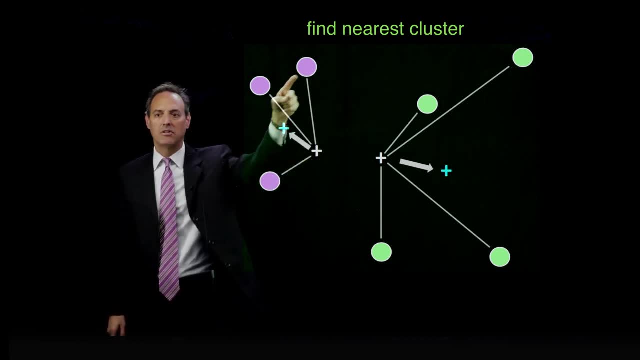 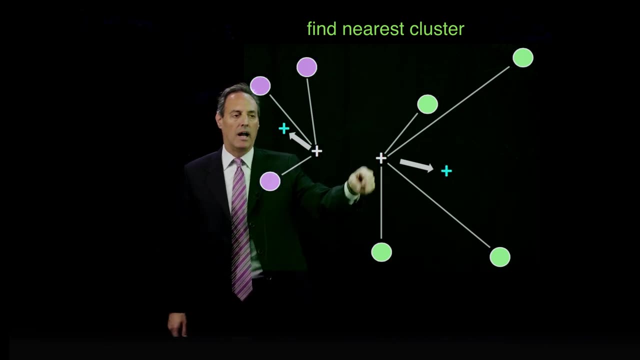 So, for instance, here: I initially picked the point here, but now, since these are my points associated with it, I move towards here, which is the center of all these points. Same thing here I have all these green points. Initially I started here, but now the center of those data points is right over here. 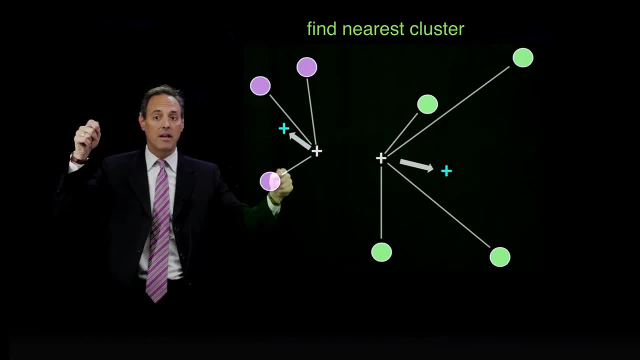 so I move those and I do it again. So now I say, okay, now that I have these new locations, everybody has to reassociate themselves to the nearest centroid point. And you do this recursively again, and again, and again until you've converged. 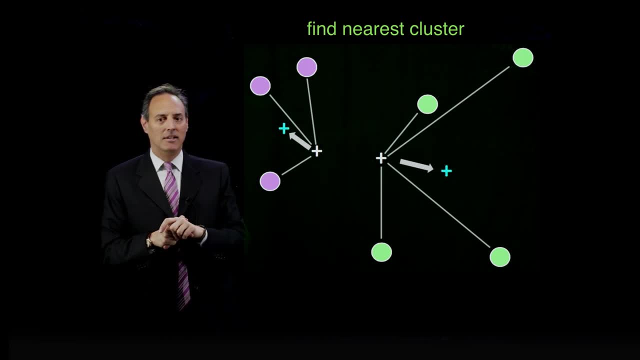 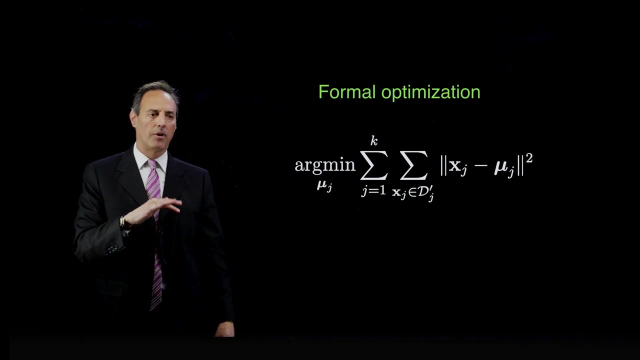 This does not mean you're right, but it does mean that you've converged to something, some kind of clustering and classification that comes out of a just straightforward algorithmic design. So that's how this thing works. It's very simple From a formal optimization point of view. 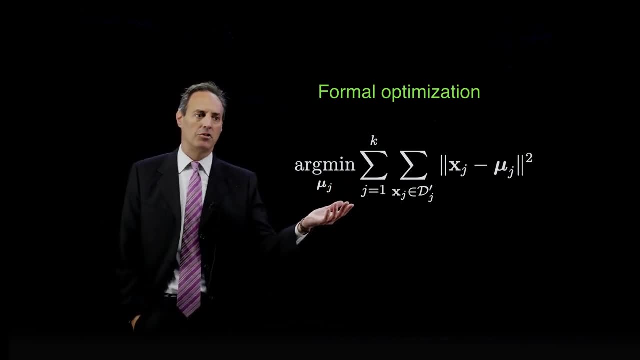 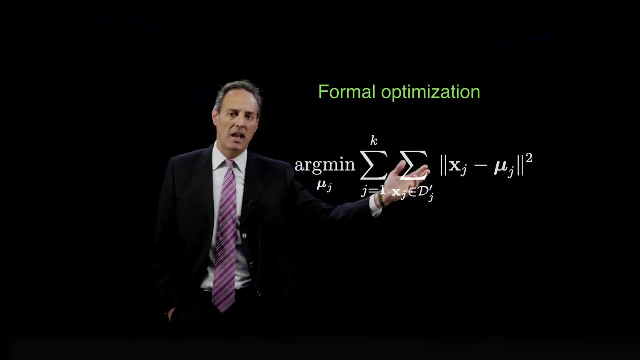 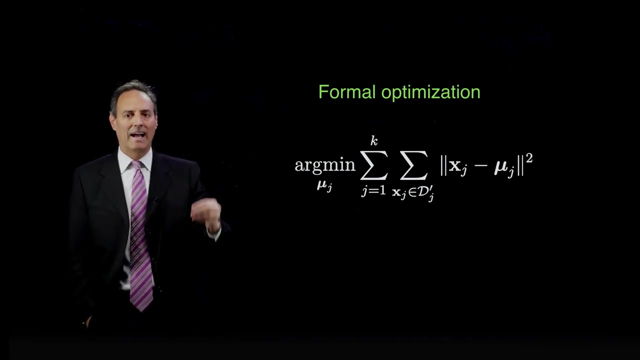 this is the actual optimization problem associated with this. What you're trying to do is minimize the distance between every data point to a central point over all of the data. So this k-means algorithm has a rigorous optimization framework. The algorithm I told you about is just to find these centroids. 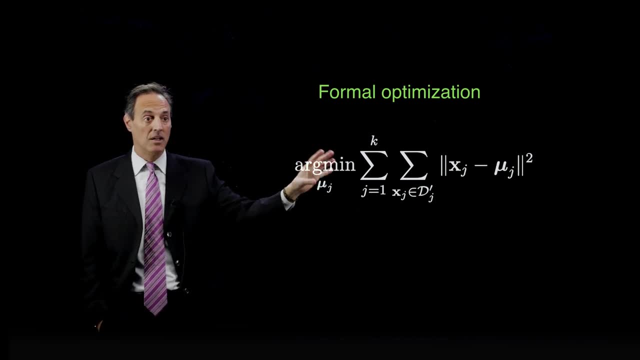 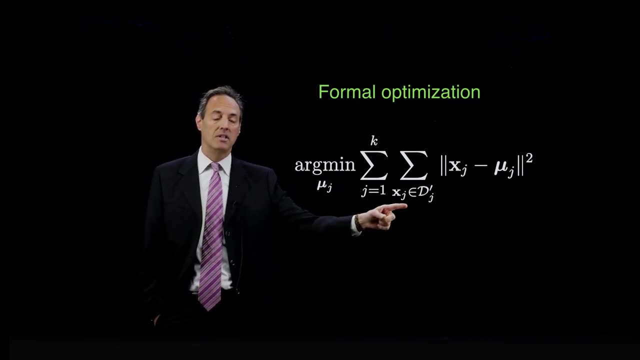 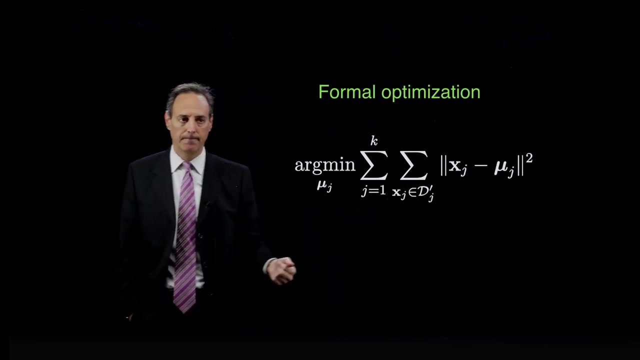 keep moving them until you've reached and you've minimized this sum here, which is the sum over the k clusters and the distance between each point to each cluster over all the data, which is the data's d prime. So that's the formal optimization procedure. 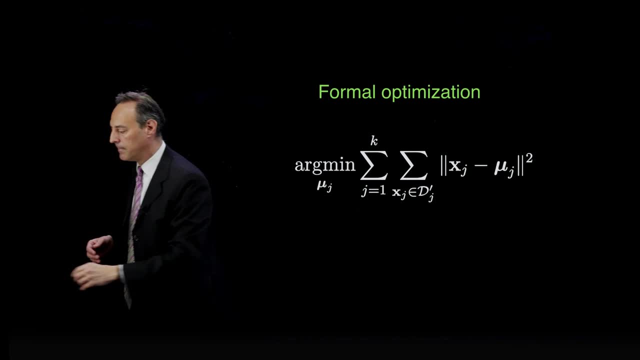 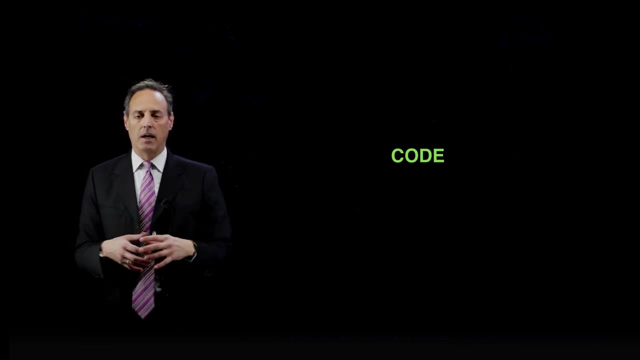 associated with this k-means clustering algorithm. So let me show you some code. We'll walk through some examples And then I just want to show you how it works. Again, the nice thing about k-means: it's really easy to implement. 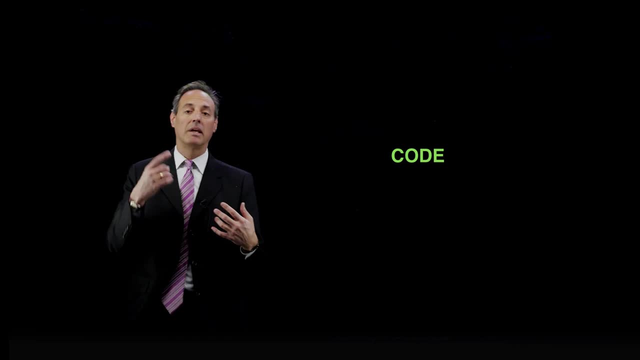 You're not making many decisions. Actually, you're making only one decision, which is you determine ahead of time how many clusters you want And you don't know how many clusters there should be because, remember, it's an unsupervised problem. 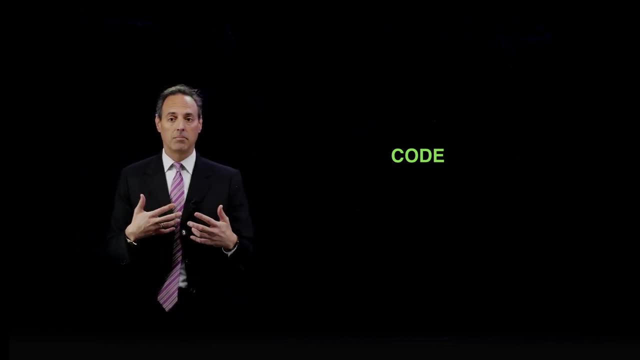 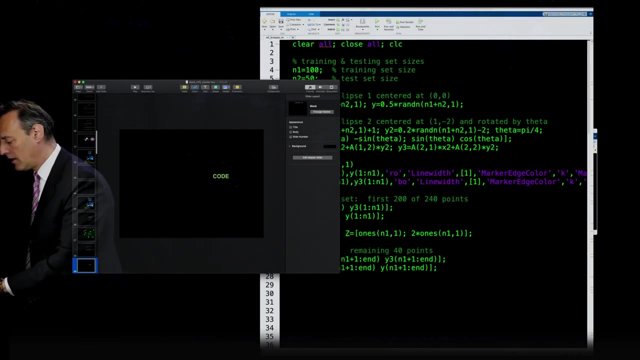 However, there are different ways- through cost validation, potentially- to pick what would be the right number, the best number of clusters, Okay, So now what we're going to do is come back to here. I'm going to put this down here And I'm first going to run this and make some data. 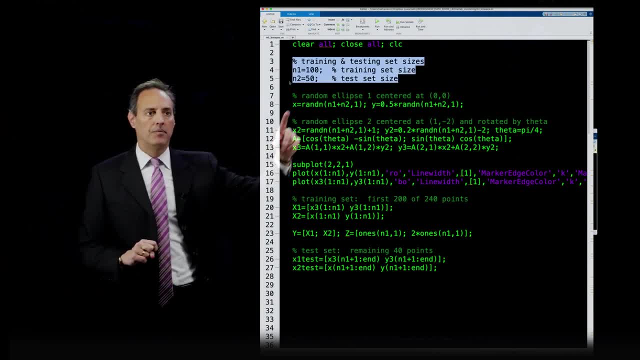 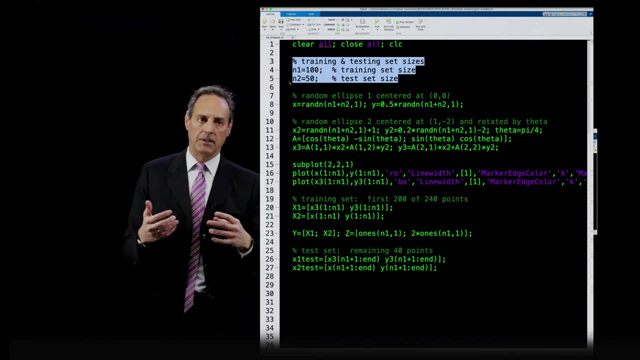 So, First, what I'm going to do is making a training set and a test set. My training set will have 100 points, My test set will have 50. So the goal here is to create- I'm going to create- two random distributions. 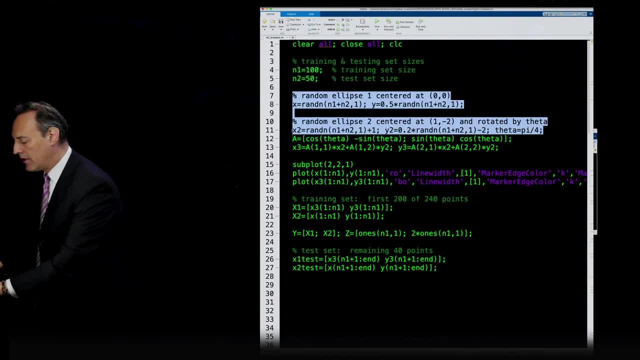 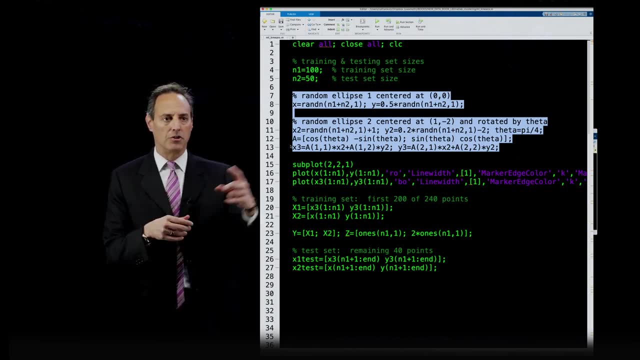 Okay, So there they are, And they're just going to be basically ellipses from Gaussian distribution, So I'm going to use the randn command here. So random ellipse, So random ellipse centered at 0, 0.. And here's a random ellipse centered at 1, negative 2 and rotated by theta. 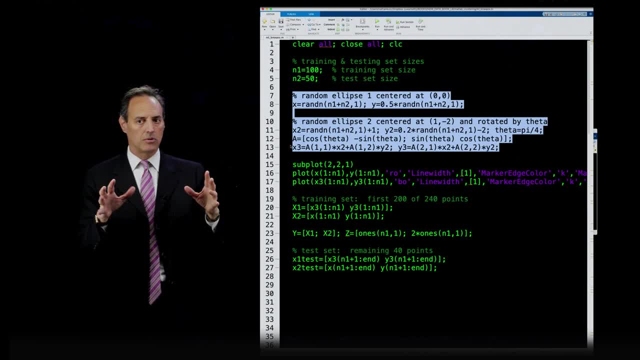 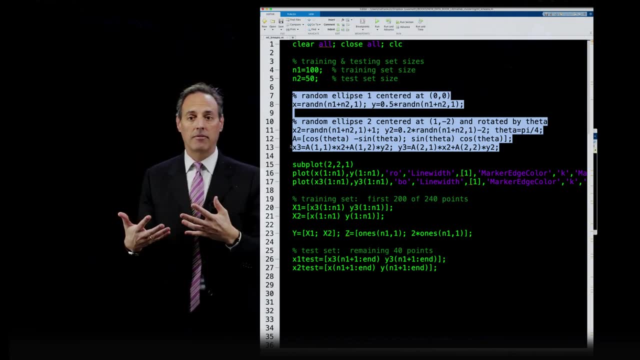 So with some angle, Okay. So, in other words, I'm going to show you what this looks like in a moment. I'm going to make two data sets. They're going to have 150 points each, And the first 100 are going to be for training. 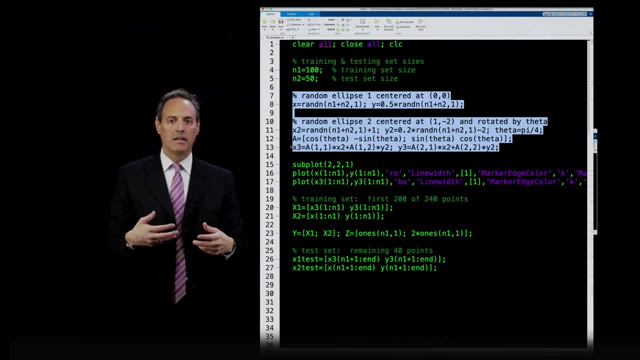 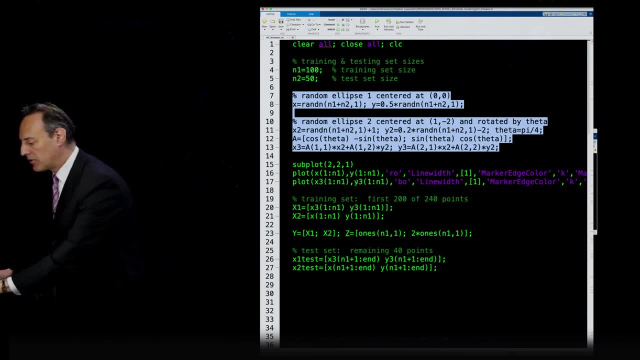 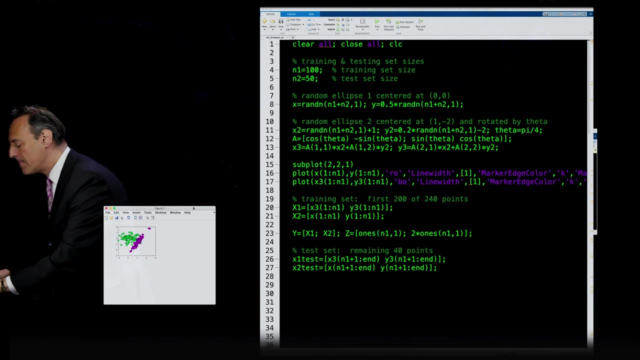 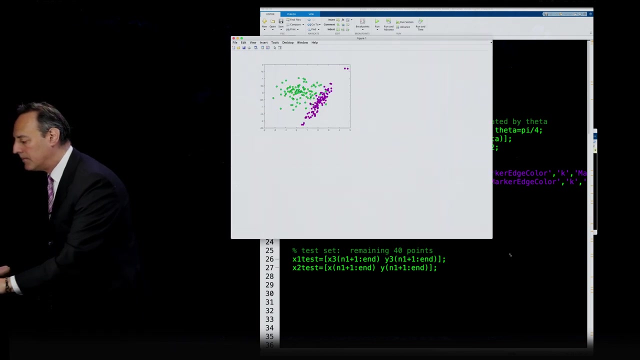 The second 50 will be for testing, So my testing and my training data will be drawn from the same random distributions. Okay, So I'm going to plot this for you to show you what these look like. Here's figure 1.. And there you go. 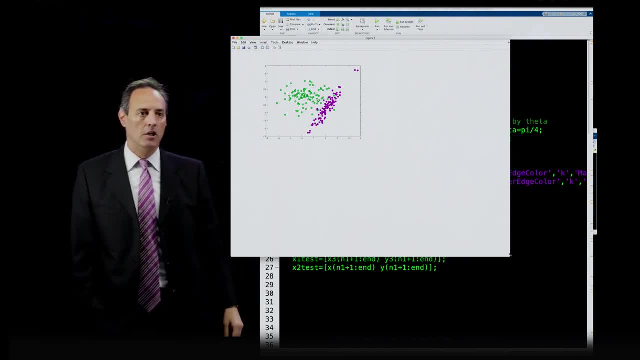 Distribution 1, distribution 2.. Okay, So one is like a stretched ellipse, The other one is just an ellipse sitting near the origin, And so what I? so? I'm making the data, So I have the truth. In other words, I've known where, I know where I got the green balls. 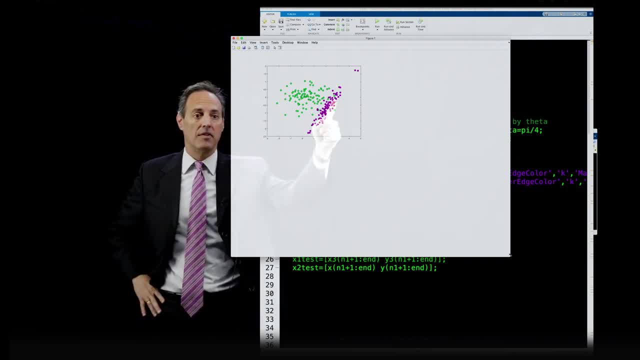 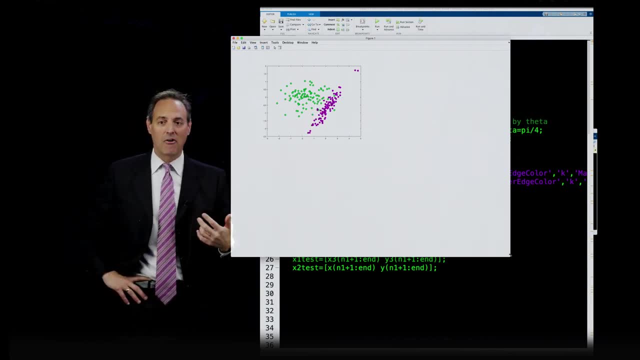 I know, I know where I got the magenta balls. I've also made it so that they do overlap right here. See, here, this is where the green and magenta balls are overlapping, So it's going to put some pressure on this algorithm to figure out what's going to go on there. 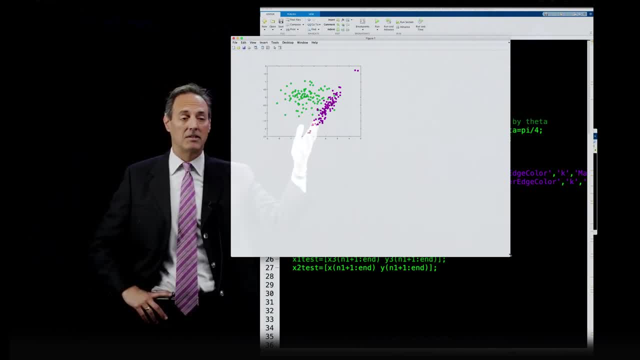 Because it's a very difficult part, because the data is mixed. So when you do clustering, what's going to happen, like, for instance, this green ball right there? That green ball right there will probably be labeled as magenta Incorrectly, even though it came from the green distribution. 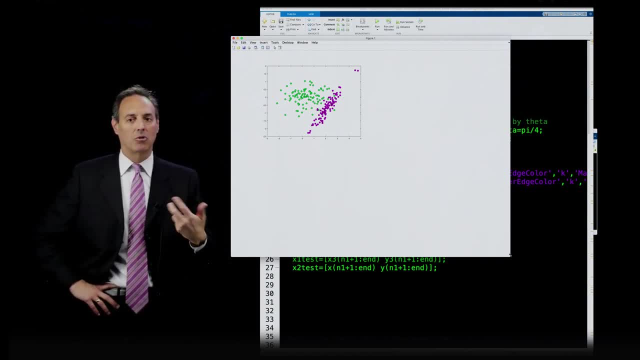 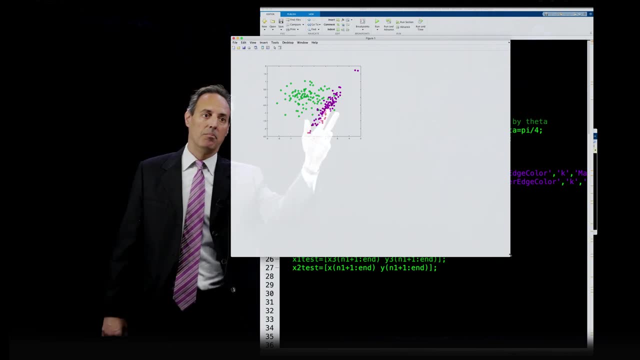 But this is the. this is the way data science goes. The point is: how many do you get correct? What's your probability of getting it correct? And, of course, your ability to get it correct depends a lot on the data set. If I would have moved this magenta further into the green region, you'd be less successful. 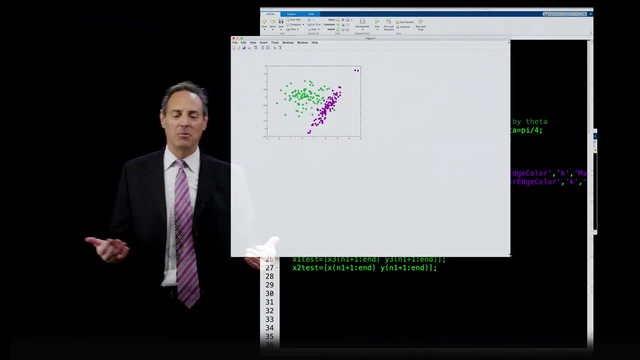 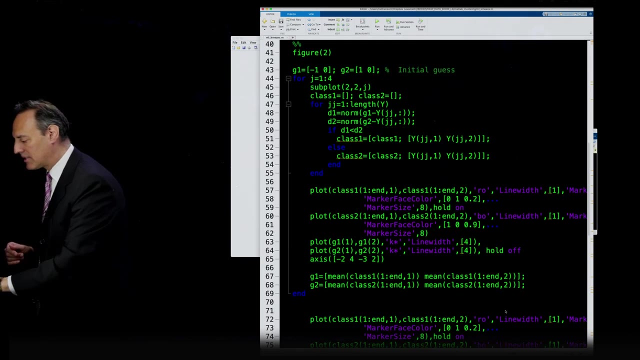 And if I move this magenta way out here, you'd almost get perfect classification every time. Okay, So the data you have really, really determines how successful you're going to be in these tasks. Okay, Now, once I have that, what I want to do is now setting up a procedure for doing the k-means. 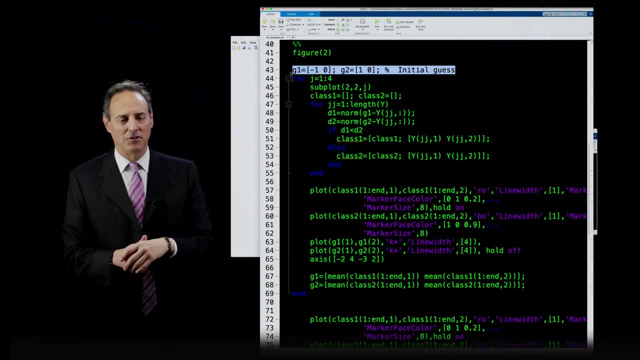 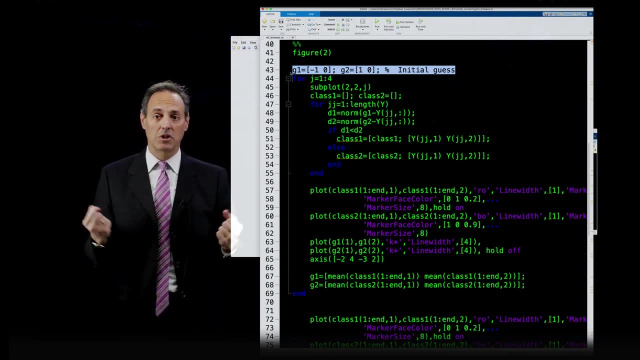 I'm going to write my own little k-means algorithm. There's one built into MATLAB that's easy to use as well. So here it is. I'm going to first of all give you an initial guess. Remember that I'm going to assume there's two clusters. 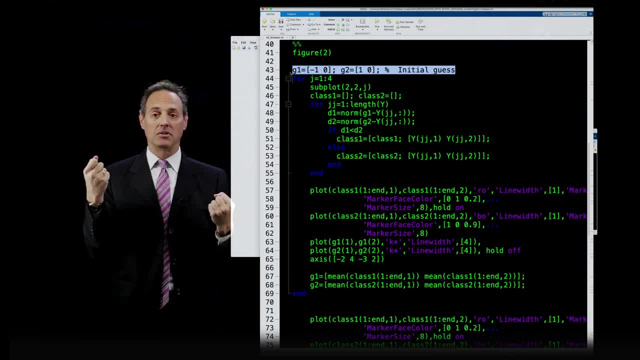 And I'm just going to pick a random position for the center of the two clusters And the way the algorithm works. I give you these two random guesses. All the points closest to this point are associated with this point. All the points closest to this point get clustered with this point. 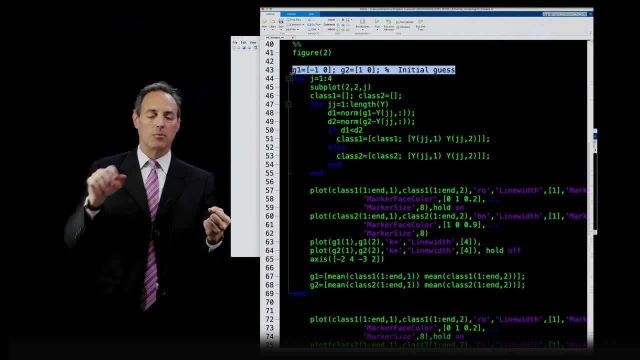 And then what I do is take all the data from this point and look at its centroid, In other words, where its center of mass is, move my point over to the center of mass, Move this to the center of mass and execute the algorithm again. 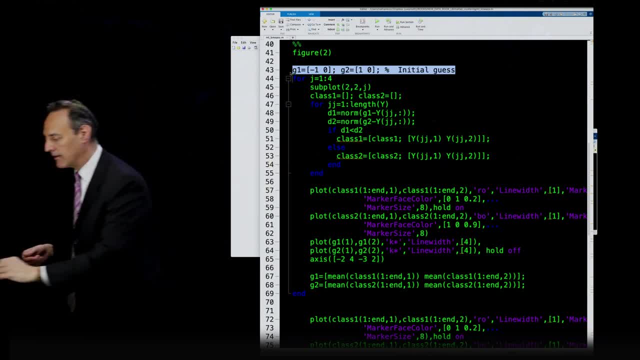 Boom, boom, boom Many times and see what happens to this thing. So this is the entire algorithm And I'm going to go through the loop four times And here's what I'm doing in looking at this loop. This is the major part of the loop. 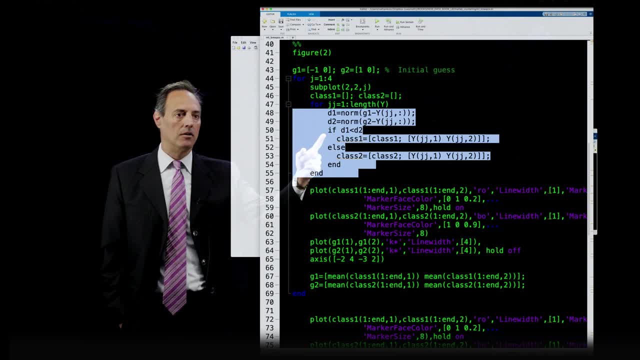 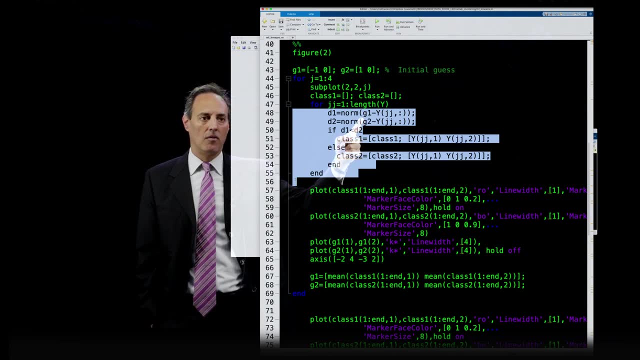 So I'm going to keep track of how things are evolving here, But what I'm doing here is looking at the norm of the distance between where my- So remember this is my guess- G1 and G2.. I'm going to look at how close I am to G1 through all my data. 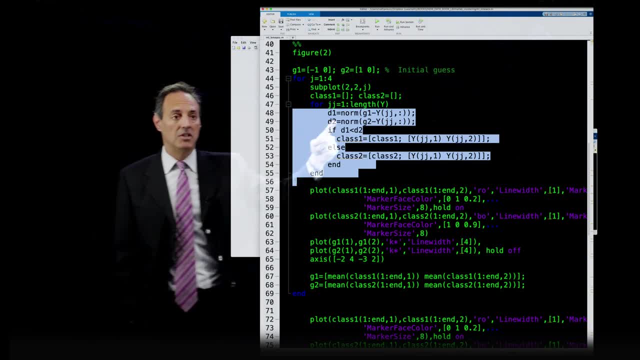 So I'm going to go through all the data and ask: what's the distance of a new data point to G1?? What's the distance to G2?? So I'm just going to say there are these two distances. I've done two clusters. 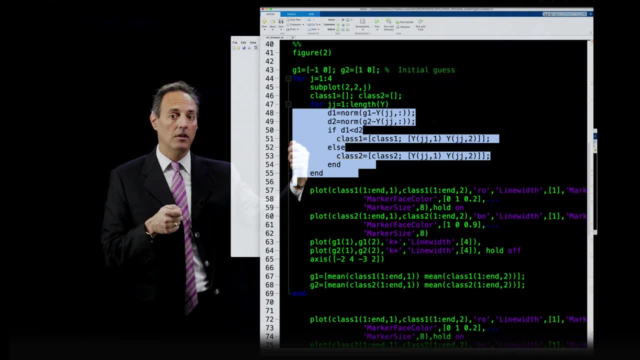 So any new data says: oh, the cluster center over here and the cluster center over there. Compute those distances And initially I start with those center points as randomly chosen And then I just ask: well, if I'm closer to one or the other. 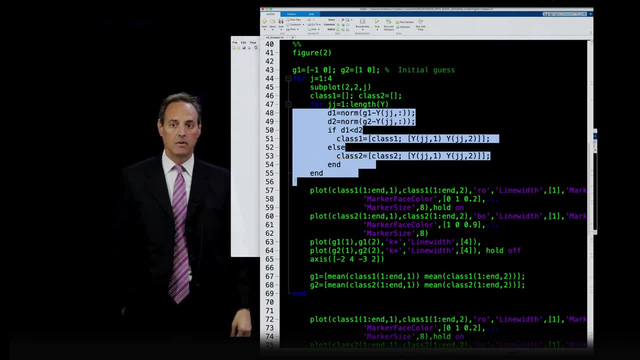 make a decision to classify myself as one or the other. That's it. So whoever I'm closest to, that's who I belong to. That's the cluster I belong to. It's simply based upon proximity, And that's what this code here does. 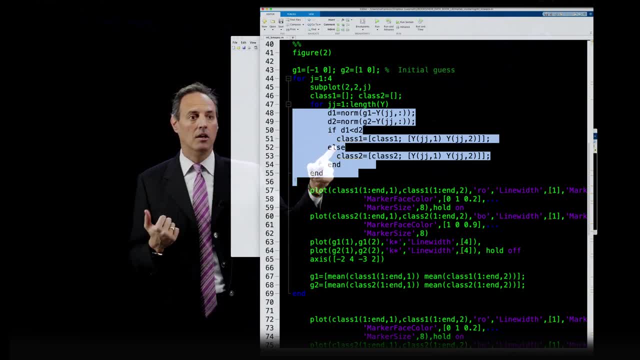 If D1 is less than D2,, in other words I'm closer to G1, or G1 is greater than D2, then I'm going to be closer to G2.. Then I'm going to classify as G2 versus G1. 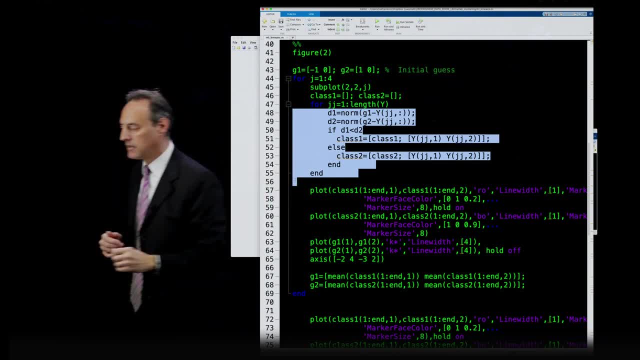 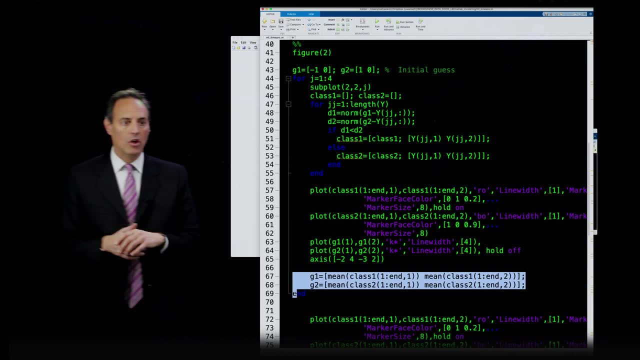 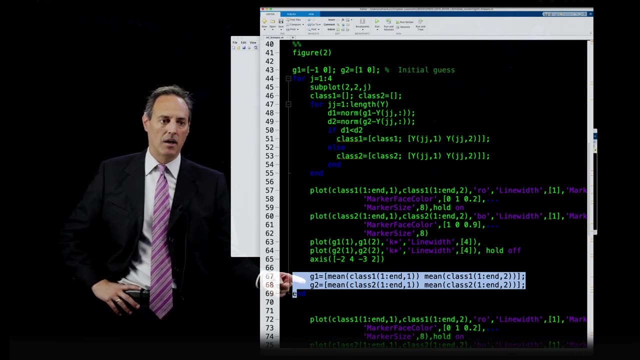 That's it. So once I've done all this and got my classifications, I want to plot some stuff here, but here's the main thing that happens at the end: Once I do this- my new G1 and G2, I just go look and see where's the mean of the clusters of class 1 and class 2.. 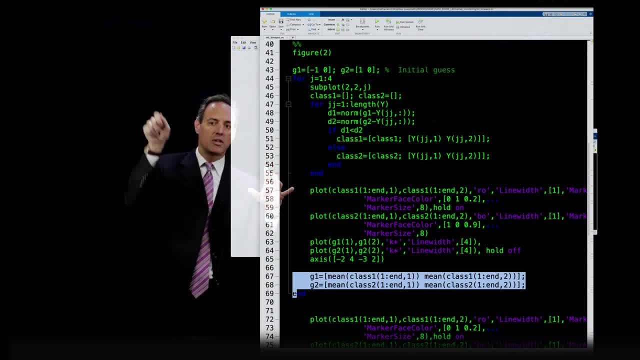 So now that I've got all the data, I go look at what's the mean value of these and what's the mean value of these. move my new G1 and G2 points to be at the mean values of those Repeat four times through this algorithm. 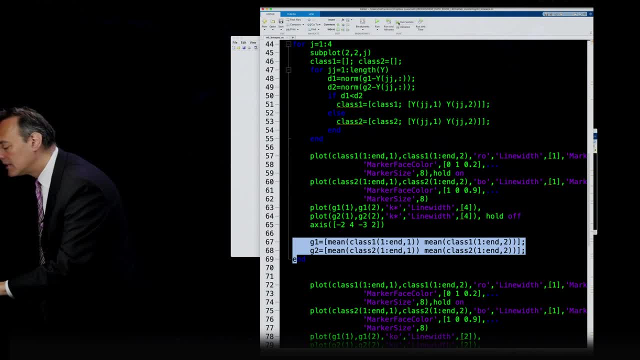 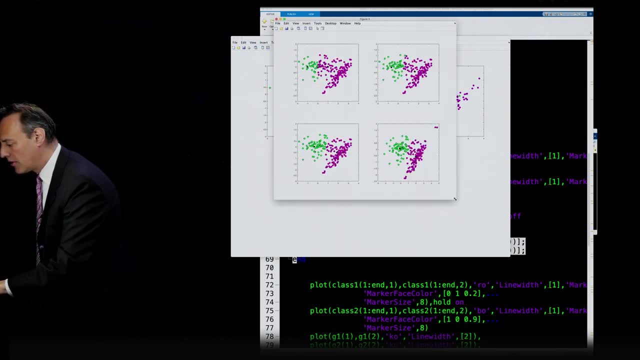 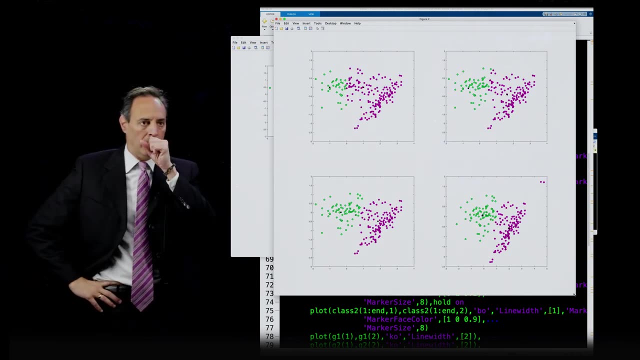 and I'm going to show you what you get here. That is the heart of it. Here it is, And what I'm showing you here is a complete diagnostic of this over four iterations. So what I'm showing you here. there's a black dot right here in the green. 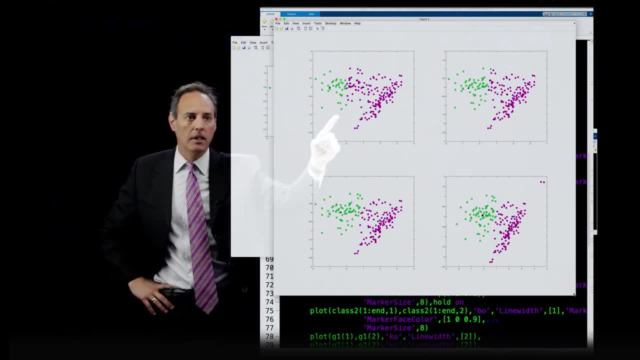 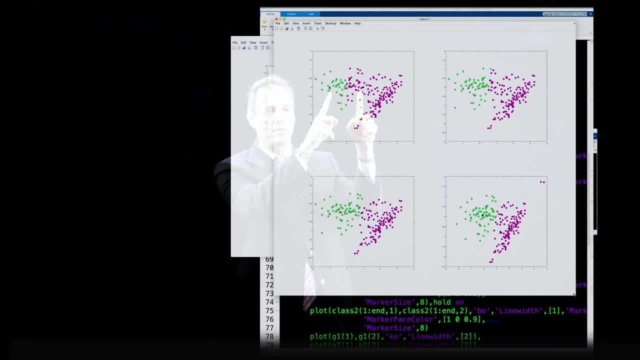 and the other centroid point, I believe, is right there. So there's these two points. So I initially picked these two points as the center points of the centroids. So notice what happens. All the points closest to this get labeled green. All the points closest to this get magented. 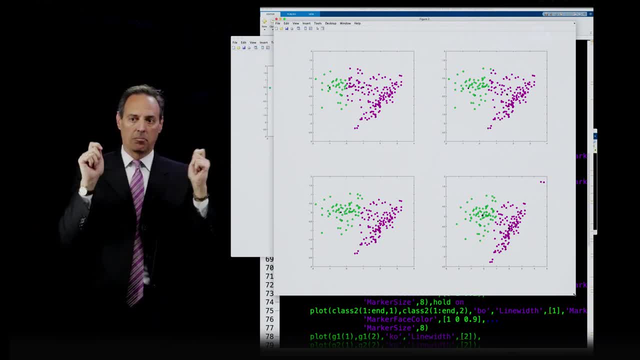 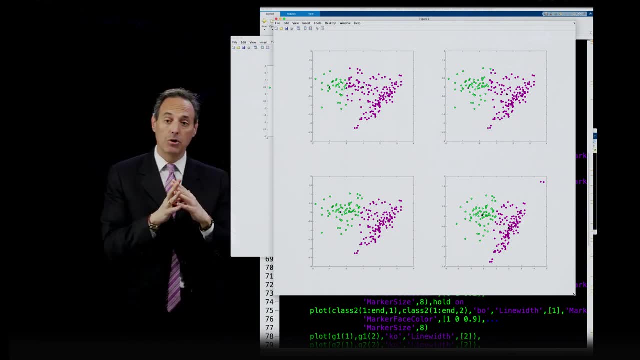 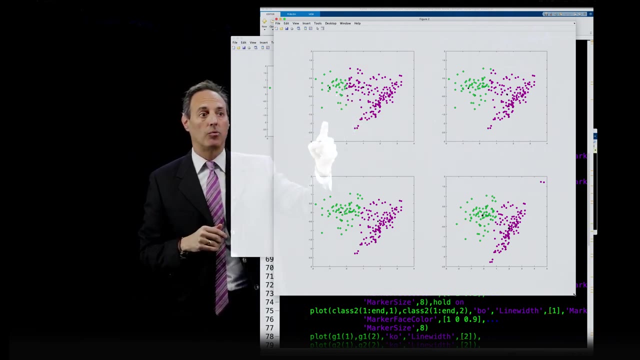 Okay, That's step one. Pick two points randomly. All the data has to belong to one or the other class. Step two is that you update the centroid. Now you say: okay, now that I've done this, figure out where the center of mass of that green is. 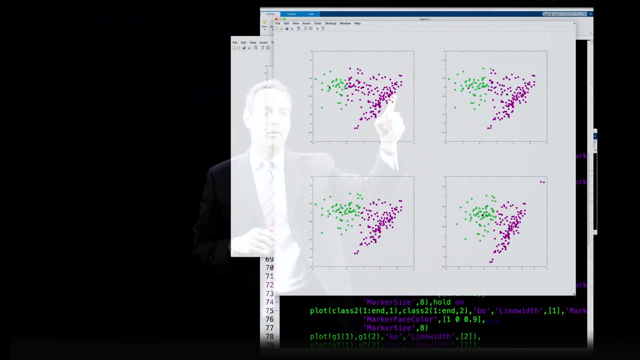 That's the new black point here. Figure out where the center of mass of all this magenta is. That's that new black point, right there. Now redo the algorithm and now notice what happens. It re-separates along this line, right there. 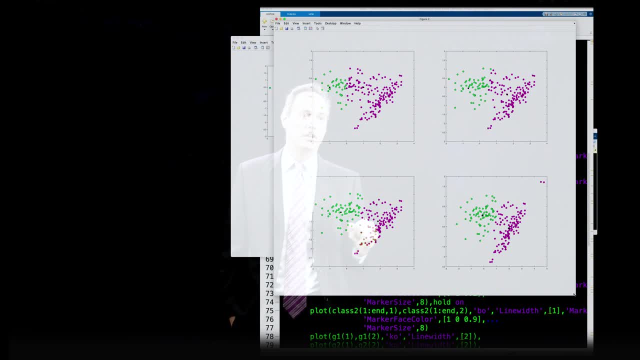 So now you have a big green cluster and a bigger green cluster and a smaller magenta cluster. Do it again And notice where the center points are. now Do it again. Here are the center points, And now you're pretty close to converged. 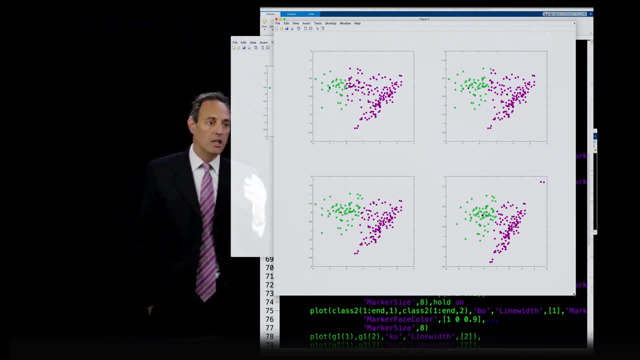 In fact, if you just keep going on this, this is very close to what will happen. So what you see is that now there's essentially a line which is, if you look at this point and this point, if you just looked at the line between them, 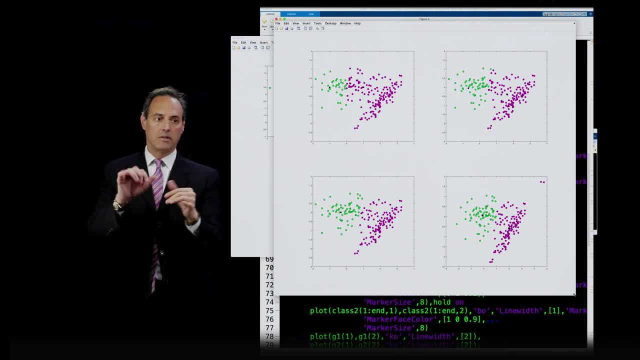 that is, that gives you the it's. basically, if you were to draw a line directly from here to the first point, to the second point, go halfway between and draw a perpendicular line this way through it, then what you have is the line separating the green from magenta balls. 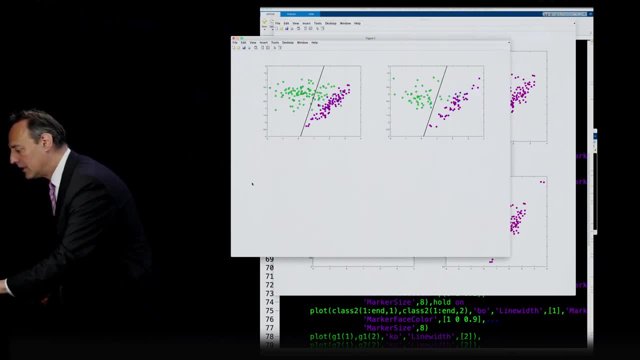 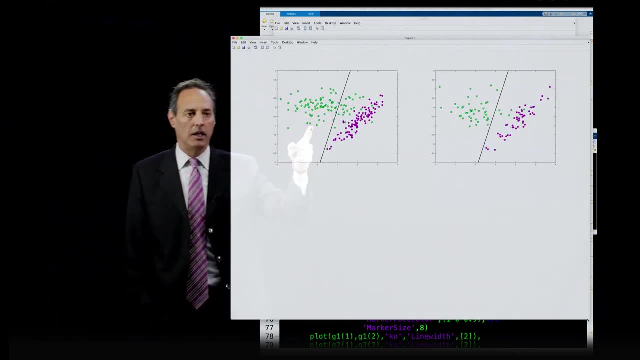 And what I want to show you is what it actually achieved. Here it is. So this here is what we did on the training data. So notice, this is the line that separates it. This is what it learns through k-means, But my actual data is now: 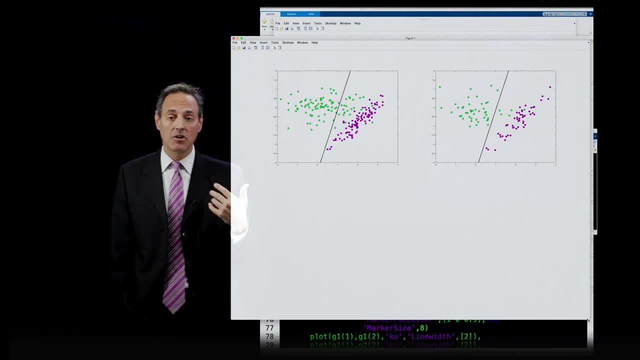 I'm showing you there in green and magenta. So it did not do the separation I actually had for the data I created. Remember, the data I created was one random distribution here, another one here and what I actually did in the separation in this k-means. 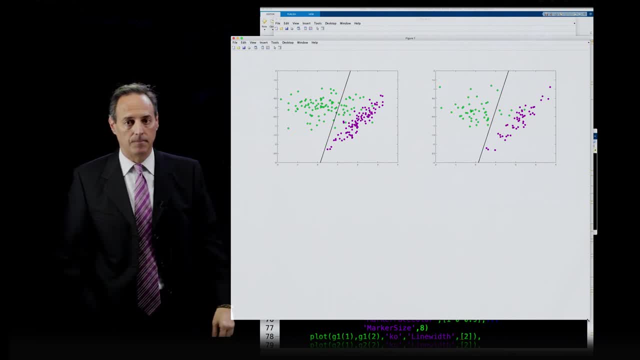 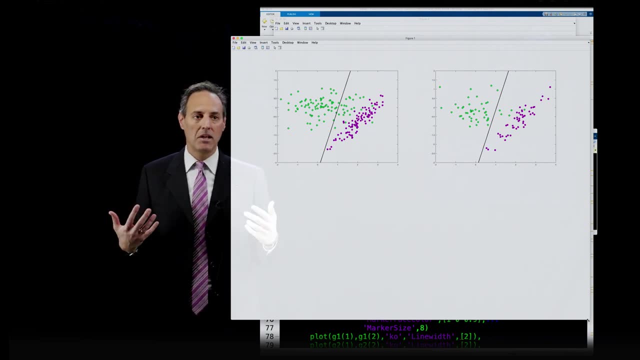 it thinks that this is the separation of the data. So you can see, that's maybe problematic. However, if I had no other information, that's still more information than what I started with. Okay, By the way, this is it. on the test data set. 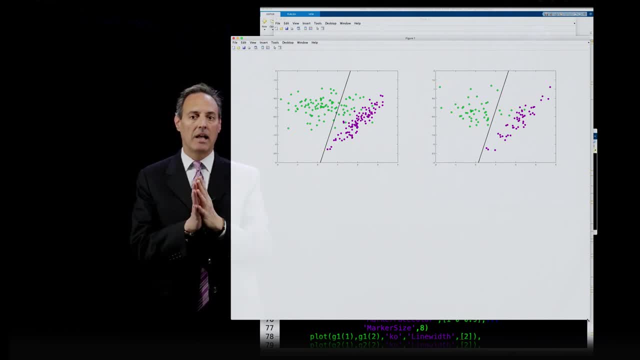 So really what I would do, I would learn this line and say, okay, with that line of classification, go classify all the test data, And this is what you'd have here, And your error actually isn't so bad: You still get the bulk of it, correct. 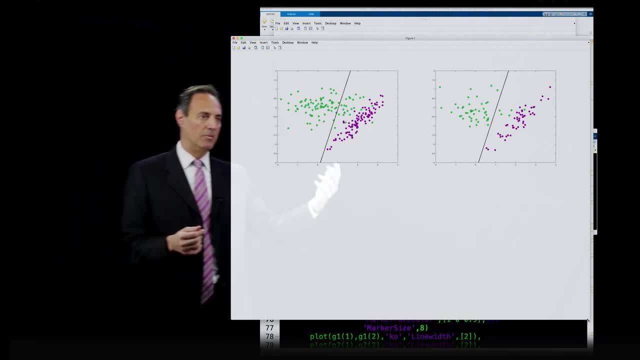 You still label most of the green balls green, most of the magenta balls magenta, and you make mistakes. And here are your mistakes: All these green balls that wander over that line Are now going to be misclassified. So the nice thing about k-means: 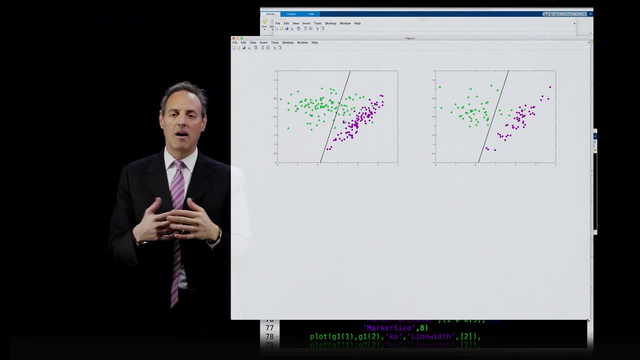 it's super simple. There's not much thought you have to put into it except for picking the number of clusters. It's just execute the algorithm Okay, Sort of. I don't want to say it's brute force, but it kind of is just brain dead in the sense you just say: 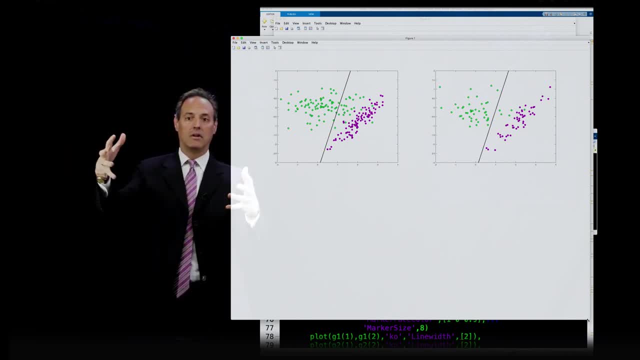 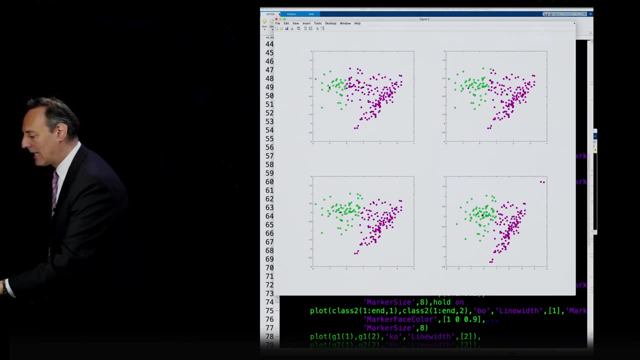 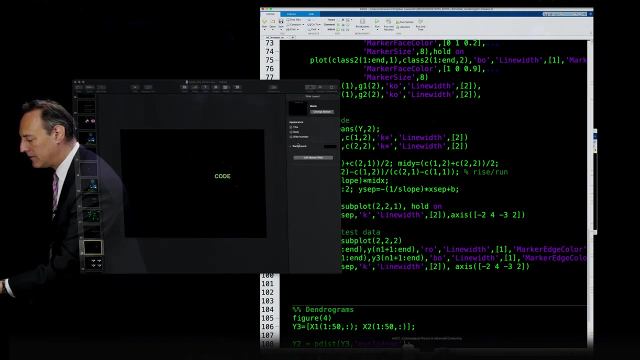 go, pick some random points, go along. So this is the algorithm. There is the k-means algorithm in MATLAB itself And one of the features it offers for you. in fact, let me come back here. Go back, All right. by the way, here's a highlight of that algorithm. 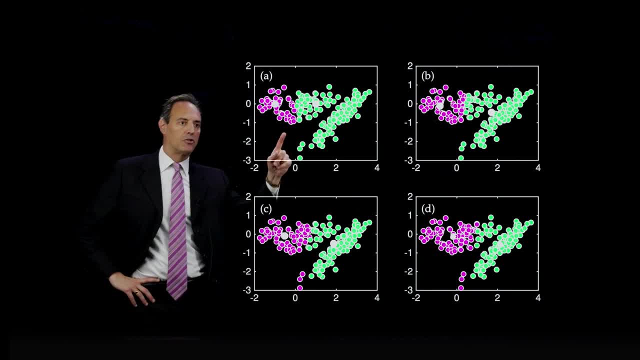 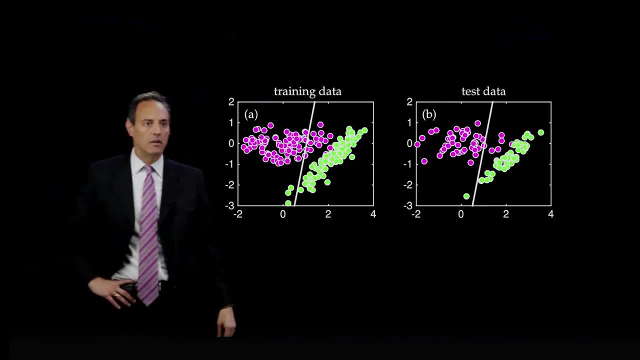 as we went through it And this is how it actually started, And you can see how that line changed and converged over there to D, And here is what you get. This is what you get on the training and test data set. Now, the one thing I want to highlight here is: 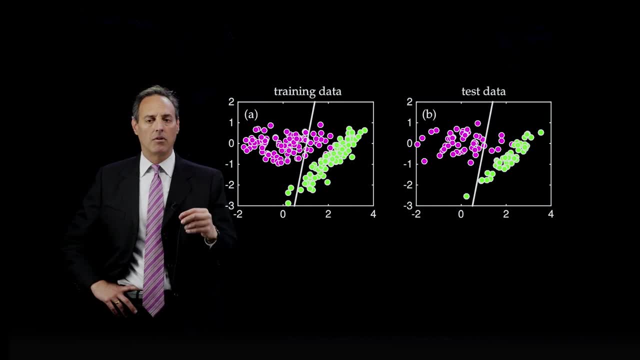 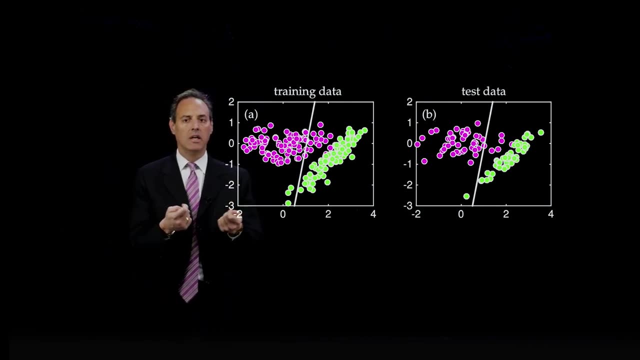 part of what makes a successful k-means is not only the number of clusters you pick, but also how you guess the initial conditions, In other words, how do you guess the initial cluster centers. So the nice thing about the k-means algorithm in MATLAB: 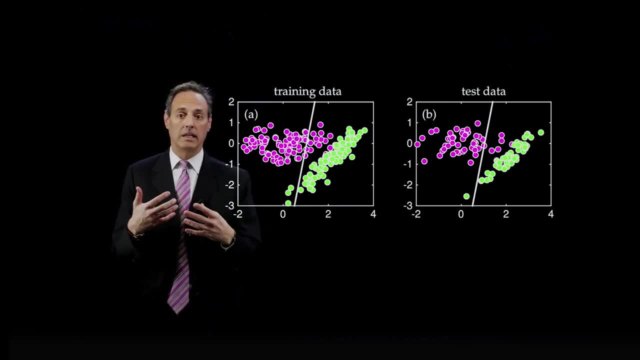 there are smart ways to do guessing. So, in fact, usually it will generate guesses directly for you, instead of you having to generate a guess. However, you can actually generate a guess. So in MATLAB, the k-means will just you give it the data, tell it how many clusters you want.